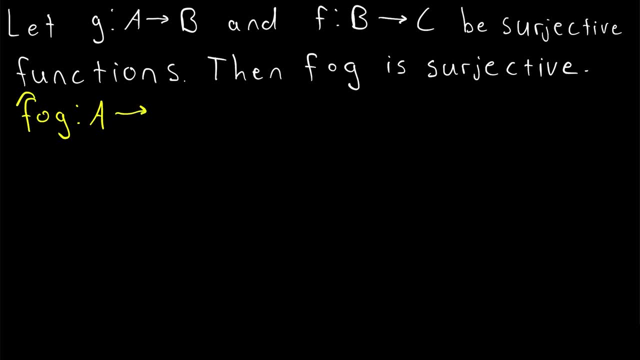 set A, and the codomain of this function is the codomain of F. That's where elements will go. So that's the set C. Let me redraw that arrow because it looks pretty ugly. All right, that's better. So the composite function F of G will take elements from A, the domain of G, then it'll send. 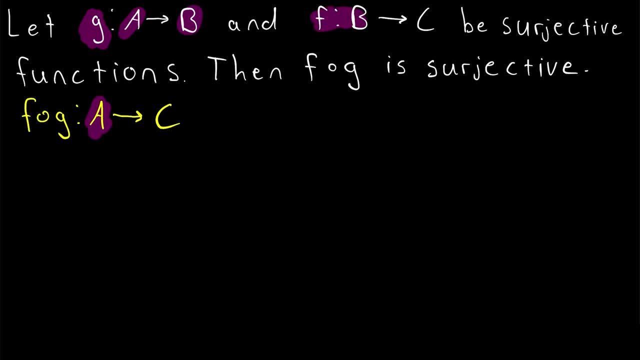 them to B, where they can then be put through the function F, which will send them to C, and that is the codomain of the function. So to prove this is surjective, we want to begin by taking an arbitrary element from the codomain. So we'll say, take some element Y from that codomain and then we'll send. 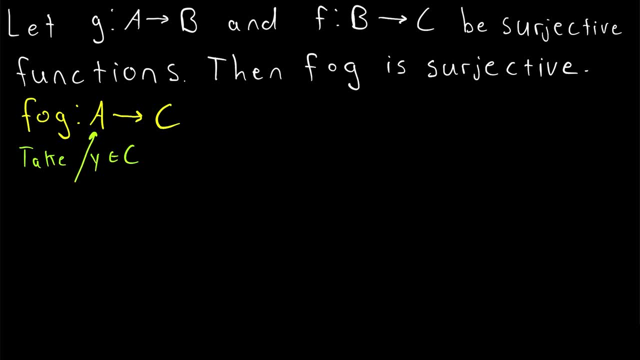 C And, of course, we want to show that there exists some element in A that this function will send to Y. So this function is made up of the composition of F and G. Which one of those functions sends elements to C? Well, that, of course, is the function F. F takes elements from B. 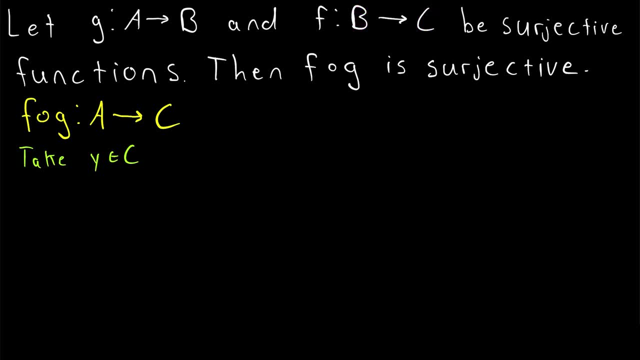 and sends them to C, And remember that C is the set containing Y. So then we might ask: does there exist an element in B that F will map to Y? And we know there is such an element because the function F is assumed to be surjective. So 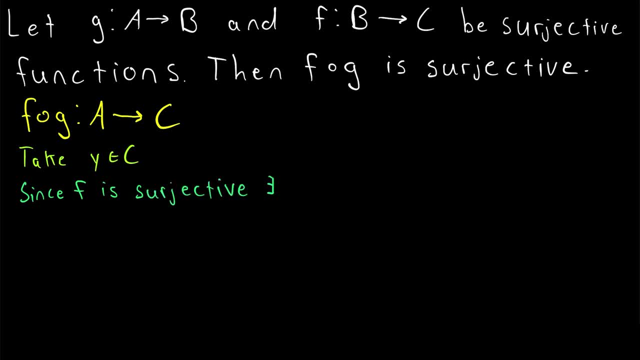 since F is surjective, we know there exists some element, we'll say X in its domain B, that's the domain of F. there exists X in B, such that F of X is equal to Y. So again, remember that we're assuming F and G are surjective functions. Thus, given any element, 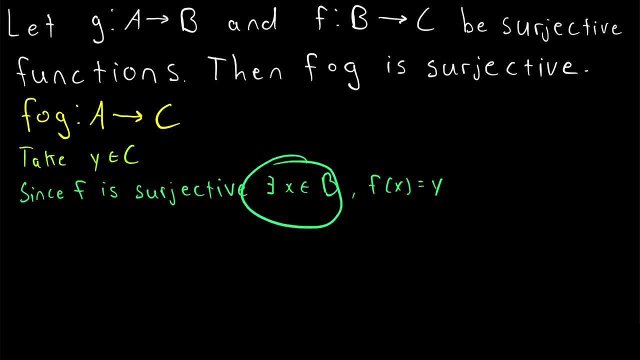 in the codomain of F. we know there exists an element in the domain that F maps to that element Y in the codomain. Alright, so X exists in the set B, And of course our function G sends elements to the set B. So then we might ask: does there exist an element in A that G? 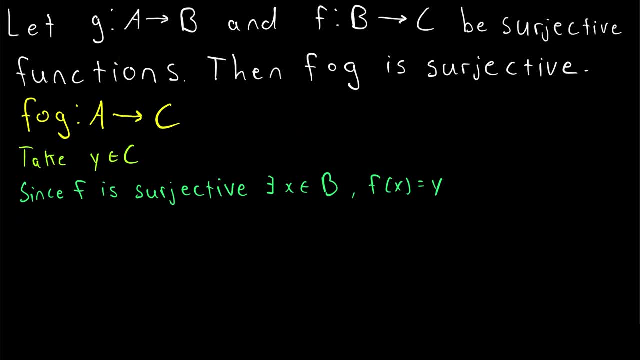 will send to the element X And just like we went over with F, we know there is such an element because G is assumed to be surjective. Since G is surjective, we know that there exists an element- we'll say X' in the domain. 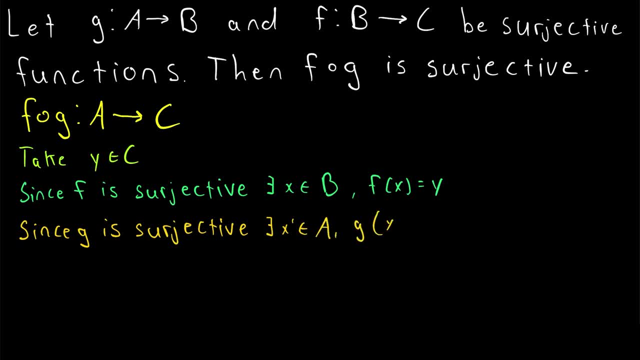 of G, which is A, such that G, evaluated at that element X' is equal to the given codomain element X. So again we assume that G is surjective. so we know we can find a domain element in A that will map to any given codomain element, And this element X' is the key to our proof. 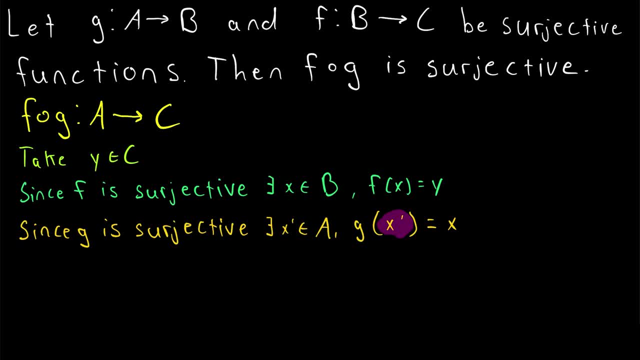 We've created this element X' specifically to do exactly what we want. So what do I mean by that? Well, plug this element X' into our composite function F. What's going to happen? Well, let's take a close look. F of X'. Remember that X' is in A, which is the domain of F. 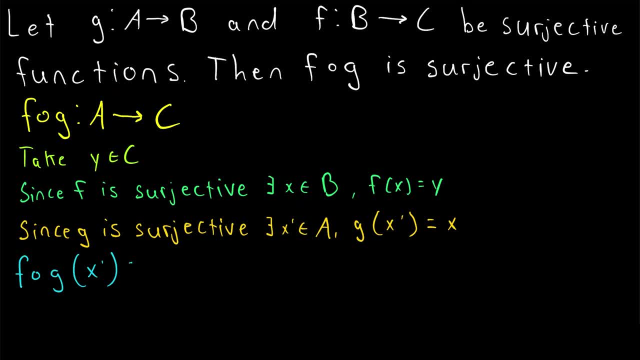 so we can plug X' into F. What is this going to be equal to? Well, by definition of function composition, this is equal to F of G'. Well, by definition of function composition, this is equal to F of G'. 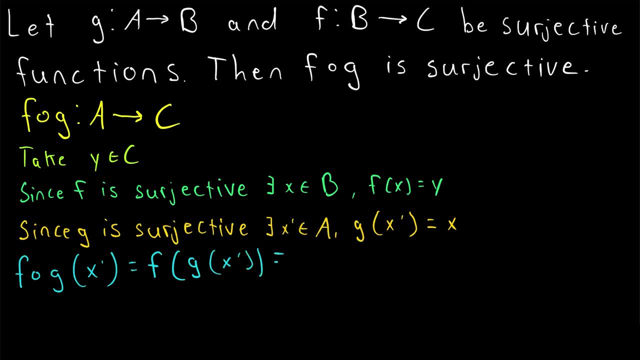 Well, by definition of function composition, this is equal to F of G' In fact, we just need F of G' of the element X'. Of course, we know that G of X' in this example is equal to X, so this is equal to F of X. that's just some substitute. 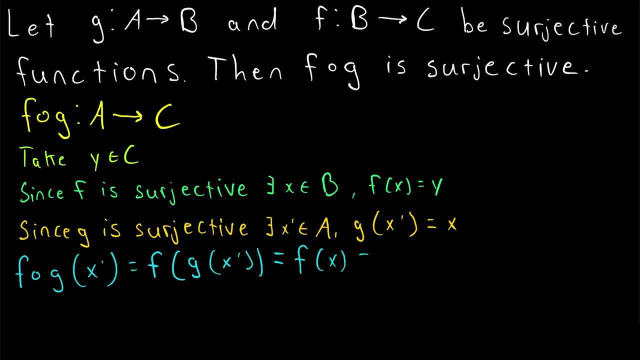 but then we know that F of X is equal to Y, so this is equal to Y. Thus, by cutting out all the middle equalities to just look at what we care about, we see that F of G of X' isго traded X' equal to Y. 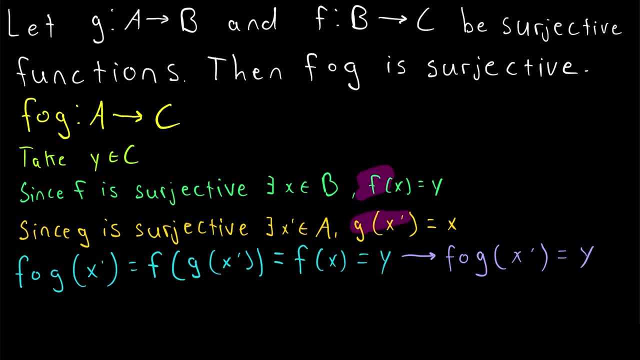 We've just shown, basically by working backwards from F to GLDQ' be equal to Y, that given any element y in the codomain of f, we can find this element x' in the domain that maps to y. Thus, by definition of surjective, we've just shown that the composition f 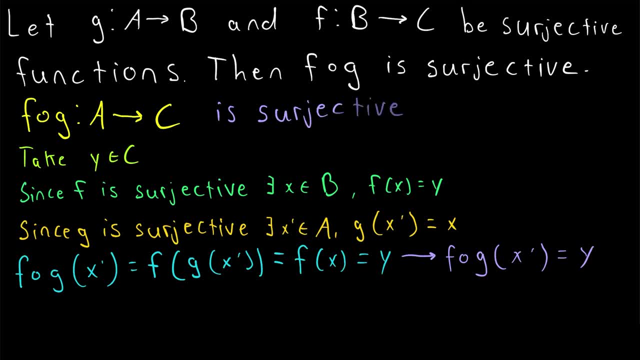 which maps a to c is surjective, which followed easily from our original assumption that the functions f and g are surjective. Now, of course, you may wonder: is the converse of this statement true as well? If we knew that f of g was surjective, would we be able to conclude that f 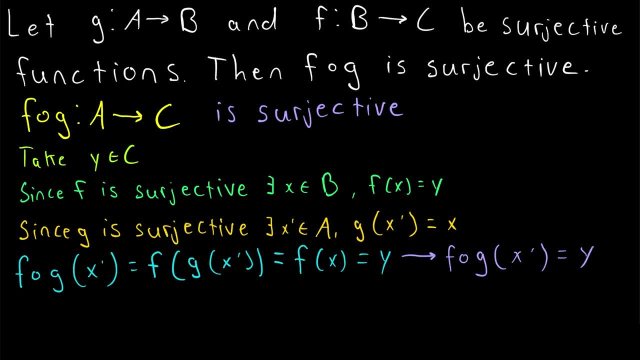 and g are surjective. Let me know what you think about that down in the comments and I'll do a video talking about it pretty soon. So I hope this video helped you understand how to prove this fun result about the composition of surjective functions. We see that function composition.